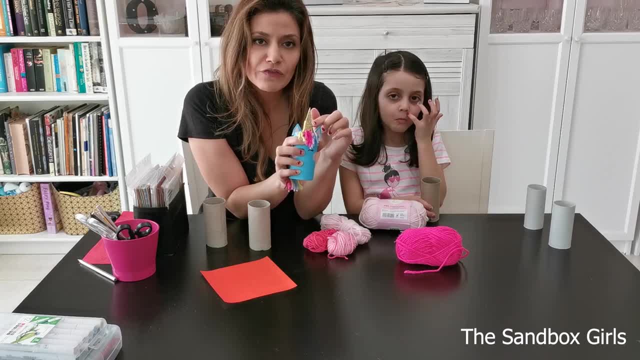 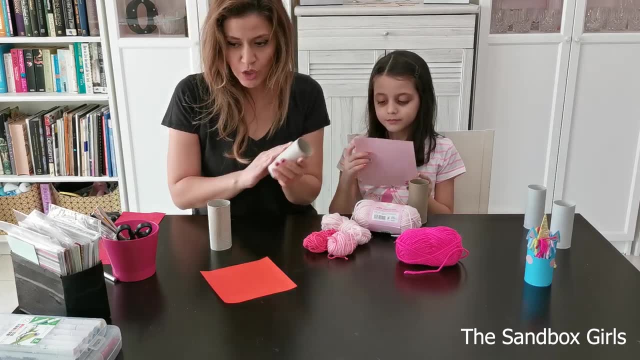 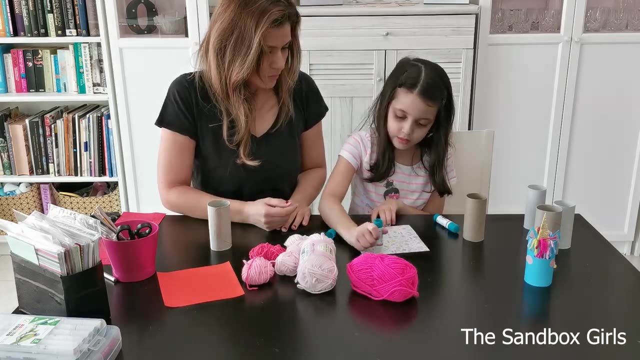 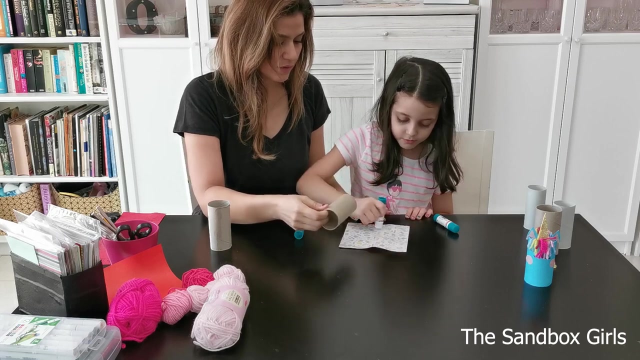 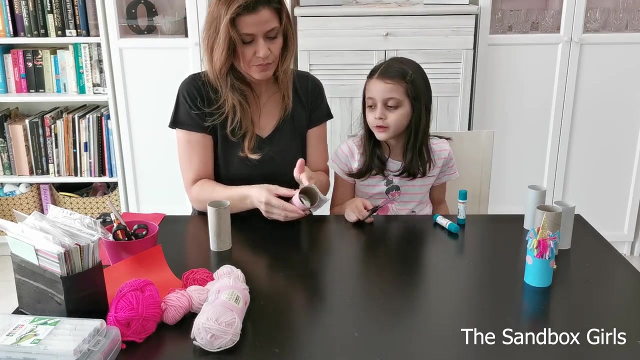 And some glitter foam paper for the horn. So here's some piece of paper. What we need to do is we need to glue it onto this horn. I want to hear it Take the toilet roll, and we do this. Now we're going to cut these bits. 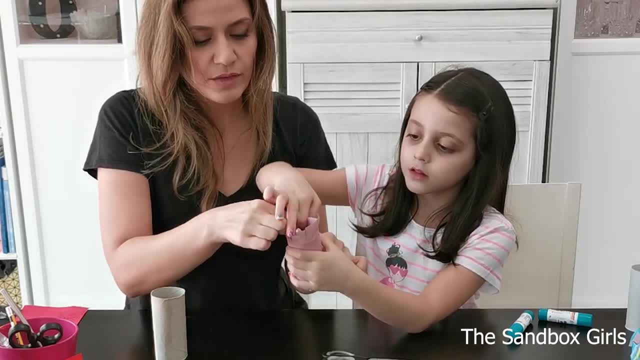 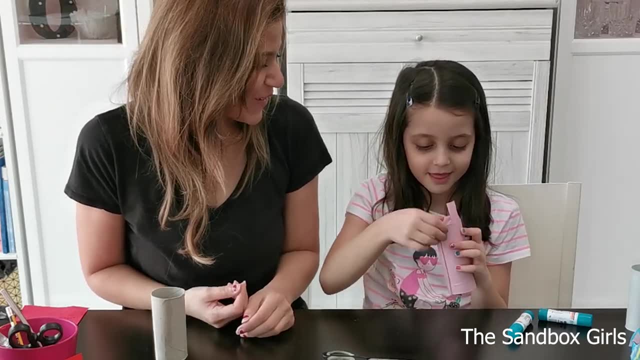 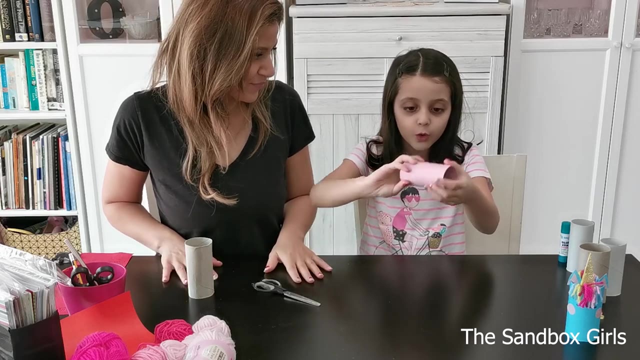 Just make sure you've got a few of these And then, since you already have the glue on, just fold them in. Do what Cece's doing: Fold it all in. So now we've covered our roll, Our roll of pink paper. 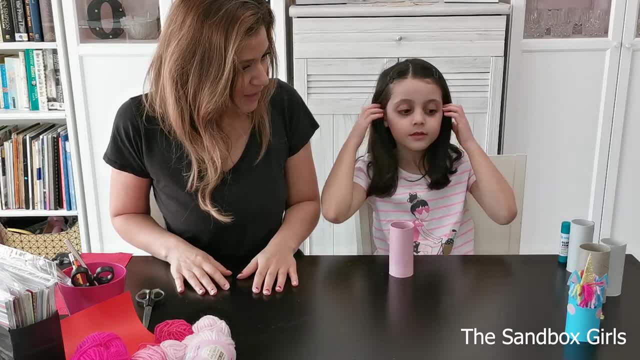 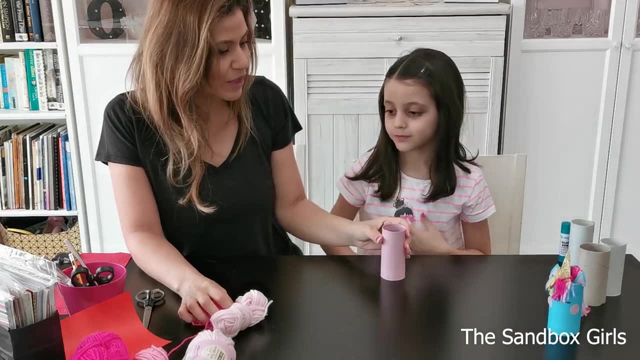 Of pink paper. All right, So now, what's the next step, Cece? The next step is to do the yarn. With this one, we went for more of a rainbow-y color, But with this one, we're going to go with pure pink. 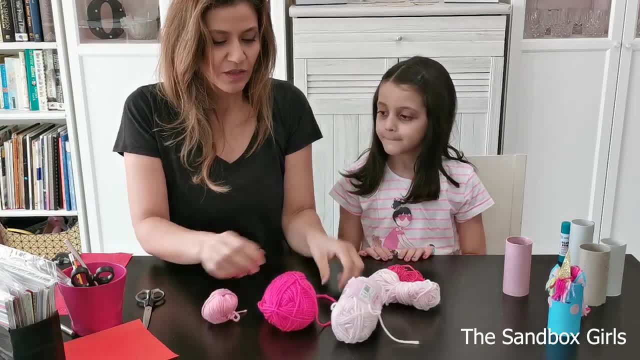 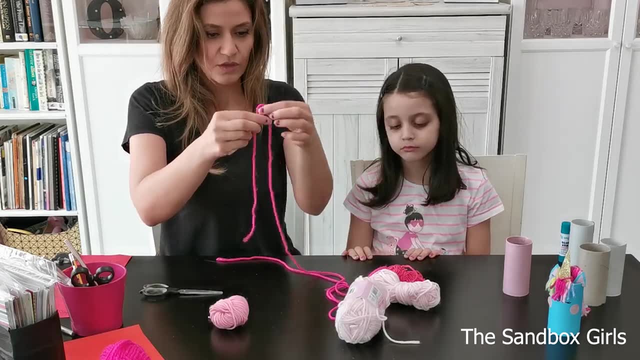 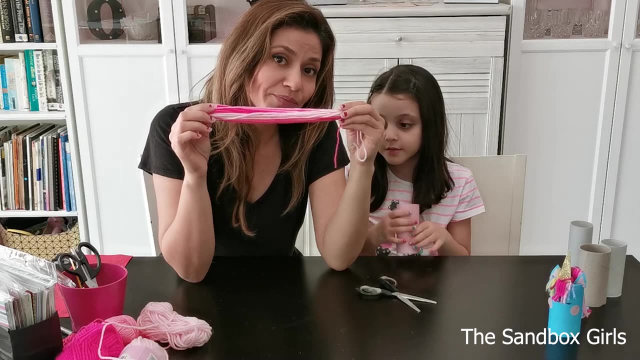 Pure pink. So I've got all these shades of pink, So we're just going to cut out a few yards of pink yarn from each. So now we've got this yarn And What we're going to do is take a little piece from here. 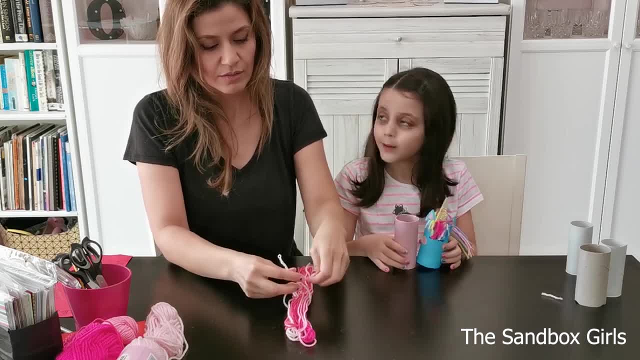 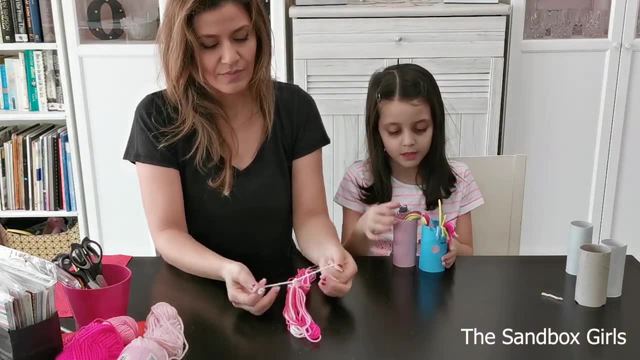 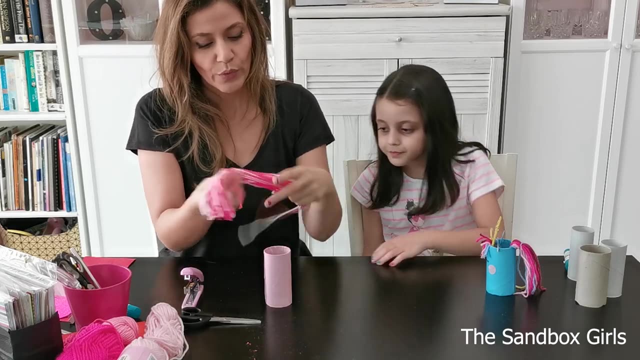 We're just going to tie all of this together, Just to make sure that they're secure. Now we're going to go ahead and give them a trim. Now that the yarn is ready, we're going to secure it to the toilet roll. 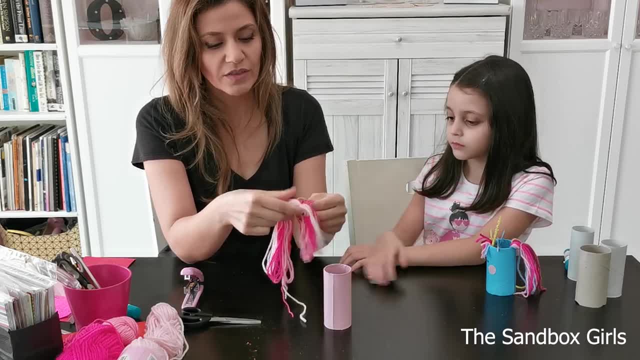 Look at the seam, And this is where the tail is going to go. Look at the seam, And this is where the tail is going to go. So this is where the long part is going to go. Now the short part is going to go right here. 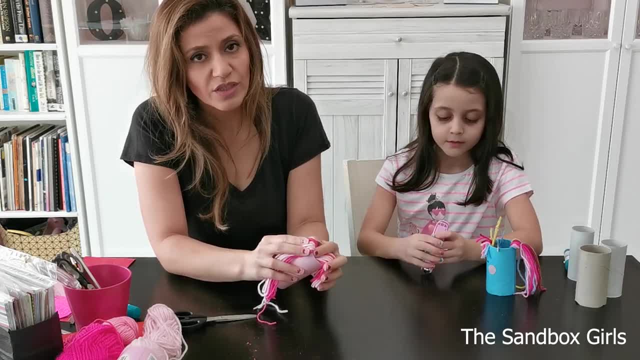 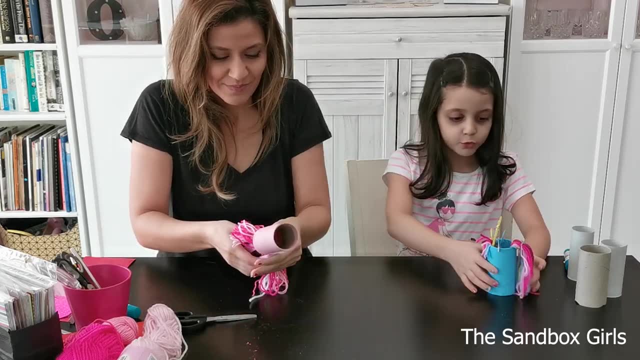 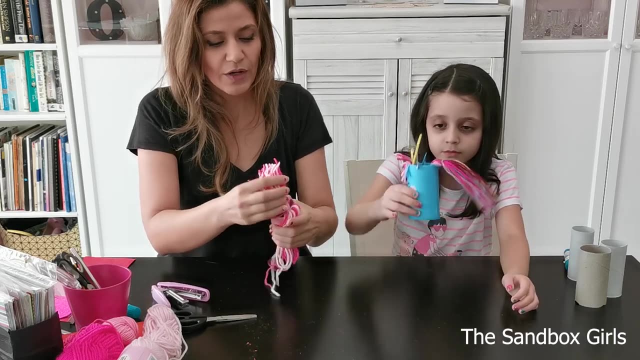 So you can use hot glue to secure it in place. But I'm just going to take an easy way and use this stapler. Stapler is much faster. Look pokey, Look Okay. as you see Now this part, I'm going to use the glue. 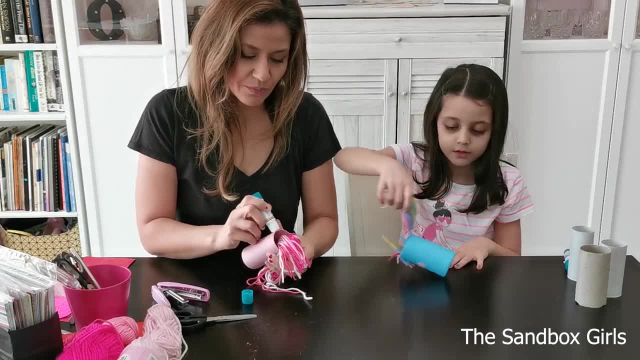 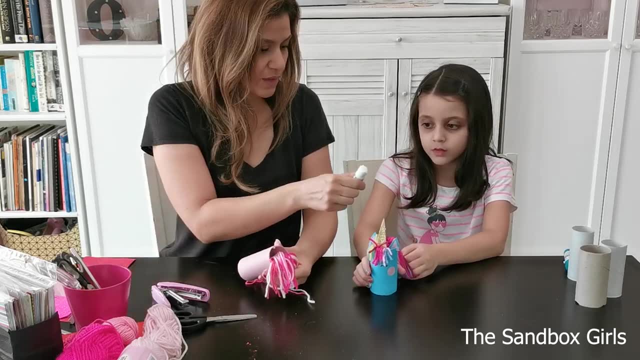 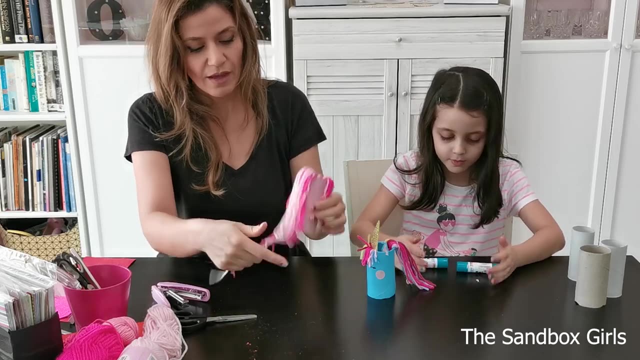 And funky glue To just secure them. And funky glue To just secure them. And funky glue To just secure them. Use a liberal amount Blue. Can you close this one please, Here In my hand. And now do you want to trim? 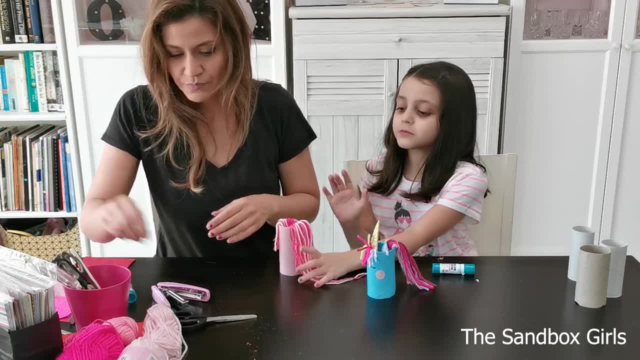 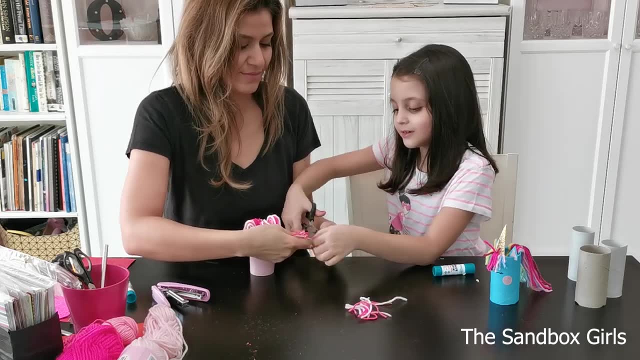 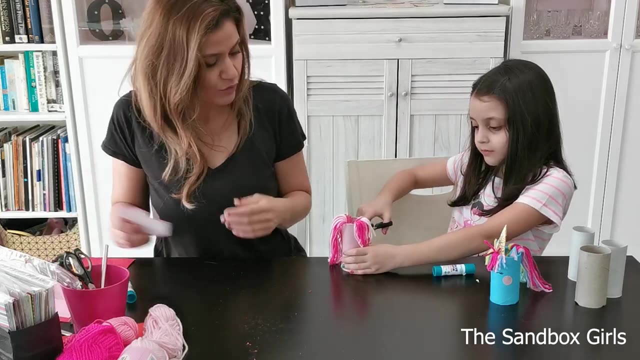 Trim Here. do you want to trim this part? Trim is my thing, Okay, see. Oh, it's so cute While Celine is trimming the mane. Whoa, whoa, careful, I'm going to prepare the horn. 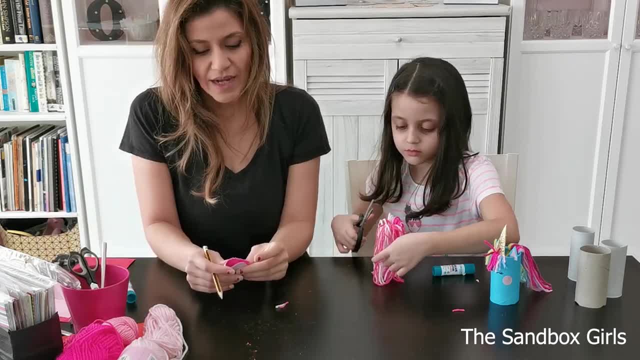 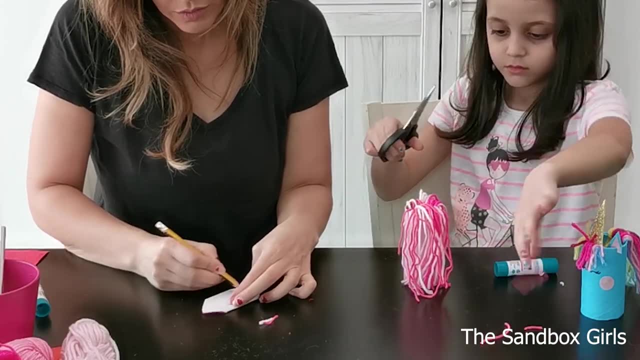 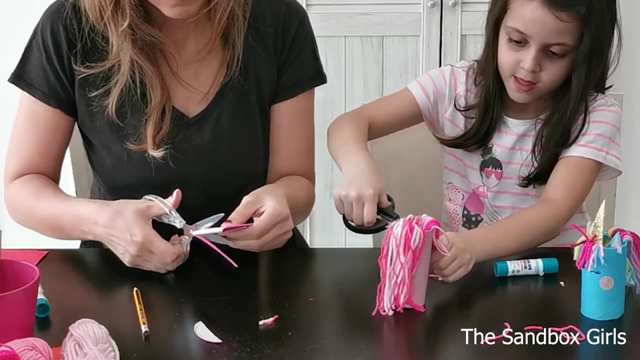 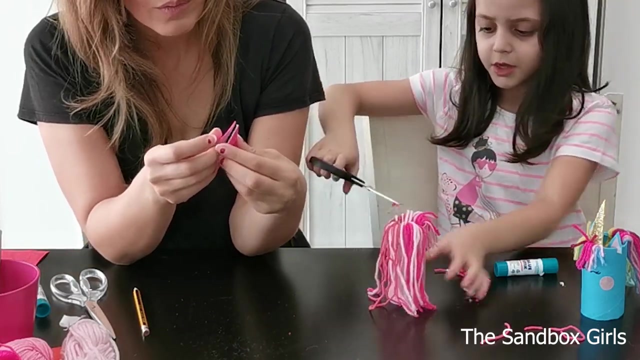 That's really easy. What you're going to do is bend this in half Because you want two sides. Just draw a horn Triangle, Take the It's on one side, Make sure you stick them. Oh my gosh, This is not good. 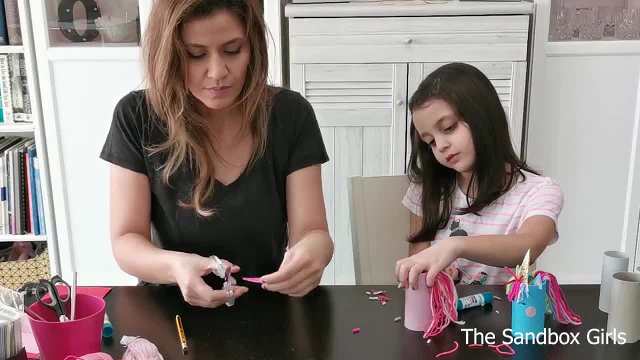 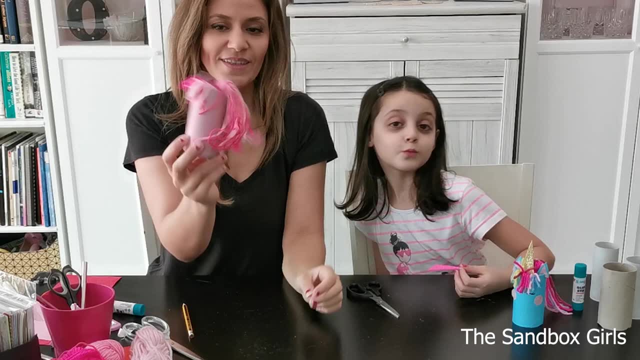 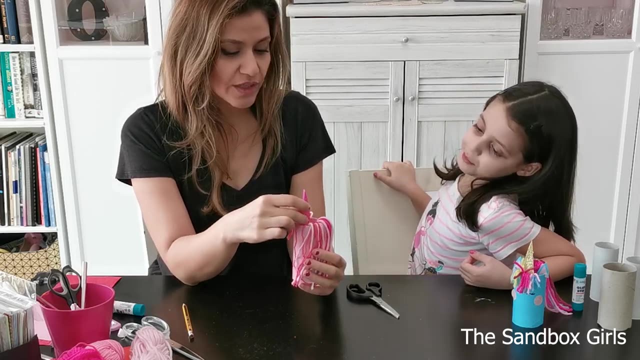 You need to trim it a little bit, It's fine. So hair style by Celine all done. Look at the eye. She's so cute. Horn is ready. What we're going to do is we're going to stick it right here. 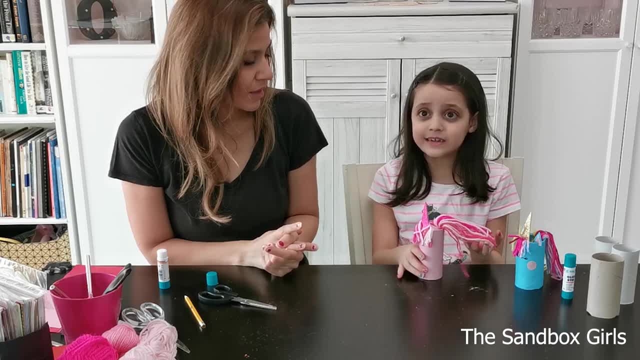 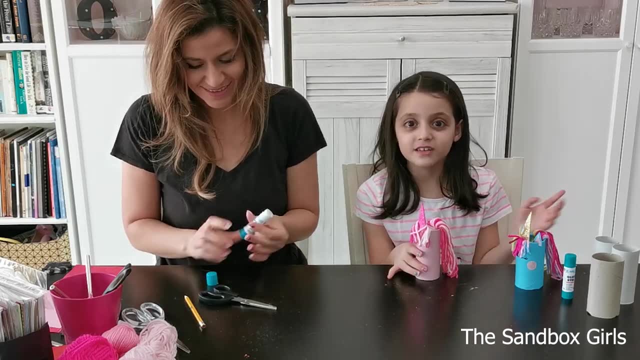 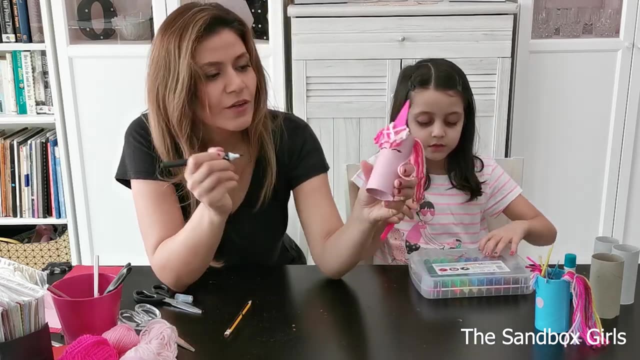 Now we're going to do the face, Which means eyes, mouth and cheeks. No, we're just doing eyes and cheeks. Oh, yeah, yeah, No mouth guys. Here we go Using the eyes and Cece's going to do the cheeks. 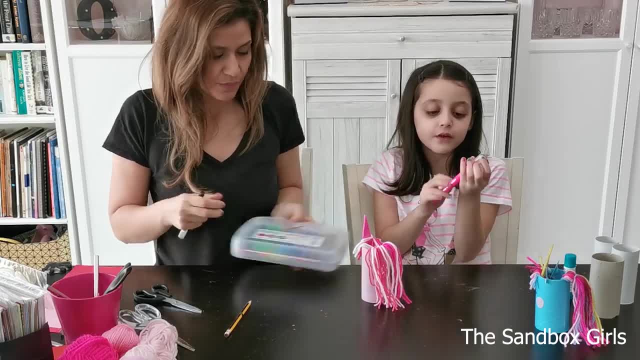 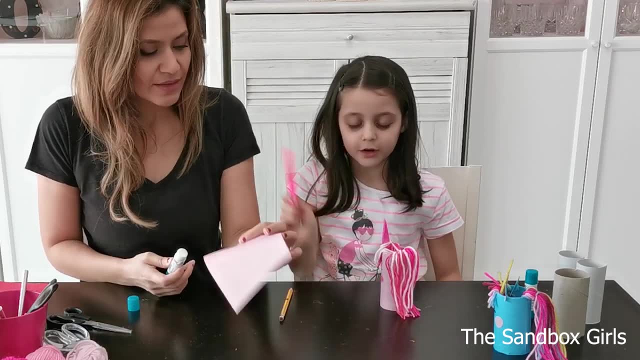 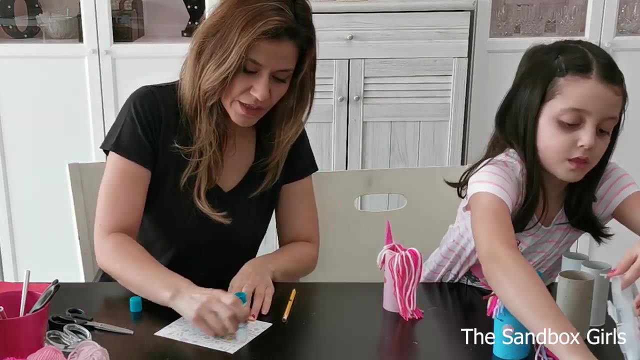 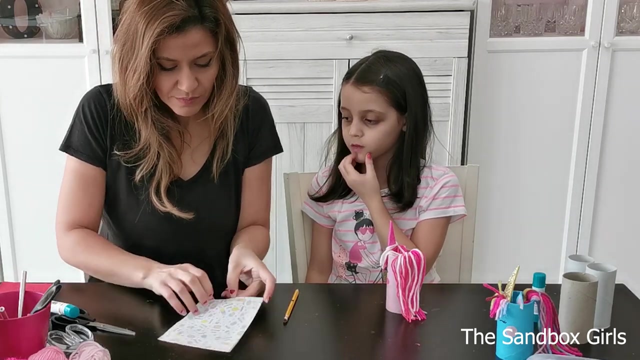 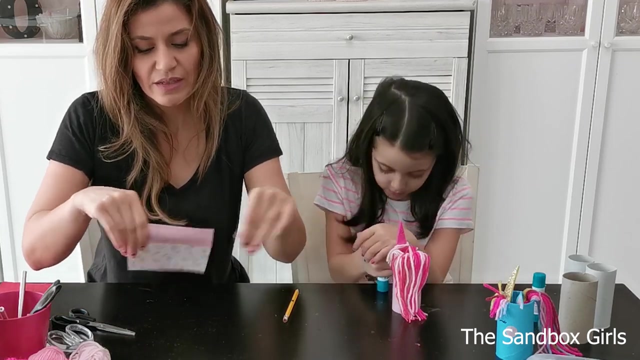 Yeah, and I'm going to use a bright and beautiful pink. Last thing we've got is the ears. Take the same paper that you used to cover up the toilet roll And just put some glue right here And then fold it. The reason I've done that is just to have the paper just a little thicker. 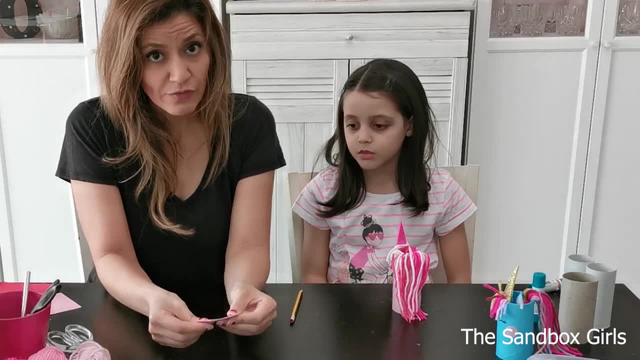 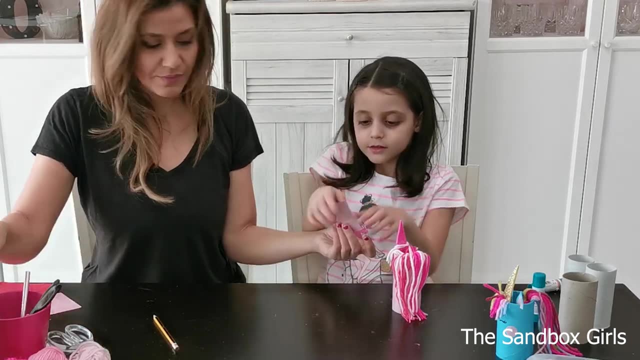 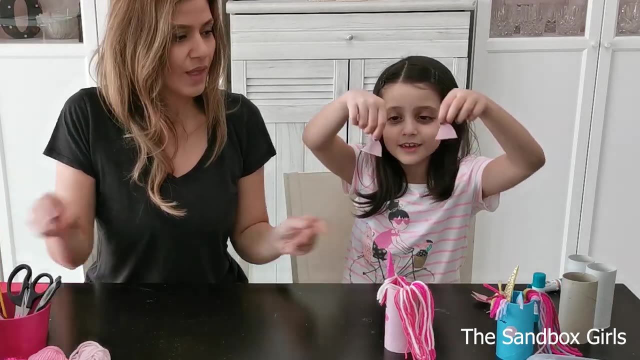 So that it will hold the shape of the ears. Fold this in half, Draw the shape of the ears, Which I love, the shape of the ears. Cece will cut it, Cut, cut, cut, cut. And these are the cute ears.